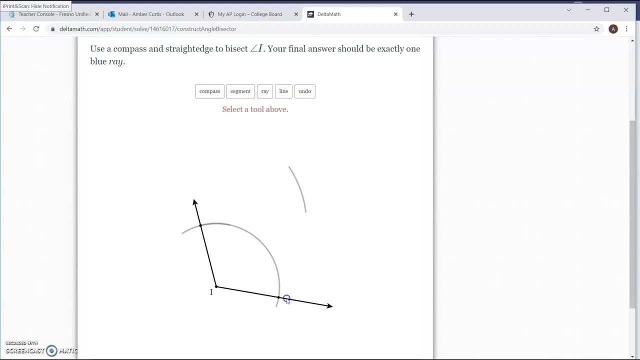 process from the other intersection. So we will click our compass, click on the other intersection and then build our circle so that it intersects the other side. By doing this, we will guarantee that equal distance that we're looking for Once we have. 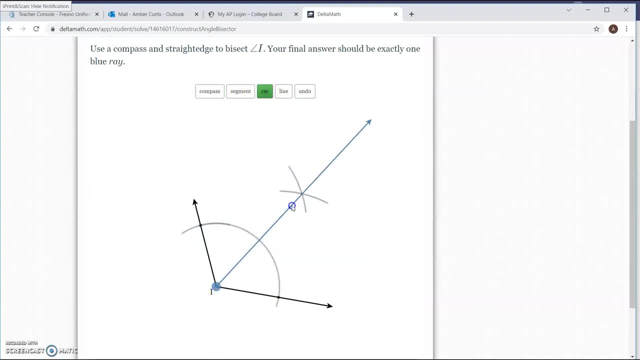 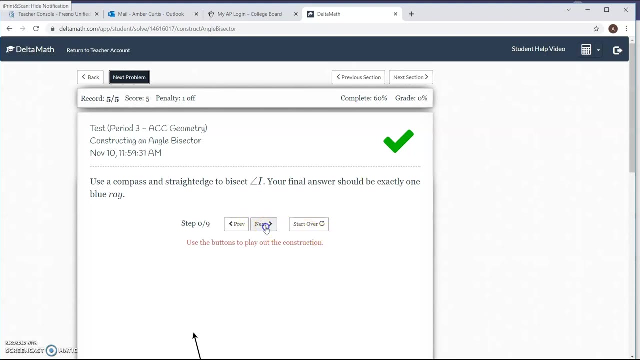 that we will create our ray, which will serve as our angle bisector, and we'll make sure that it goes through the given point. You need to make sure that you have exactly one ray. We hit submit and then it tells you your answer is correct. If you're struggling with this, it will give. 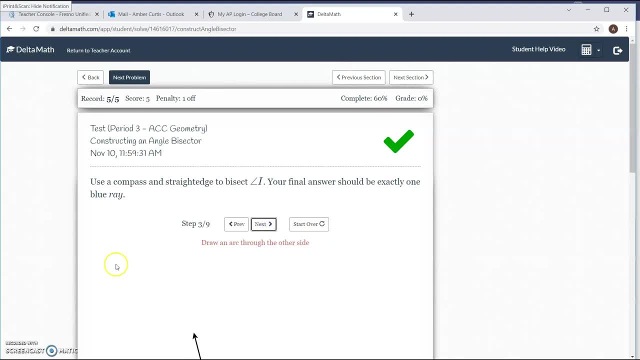 you steps and it will tell you what to do. And that's it.